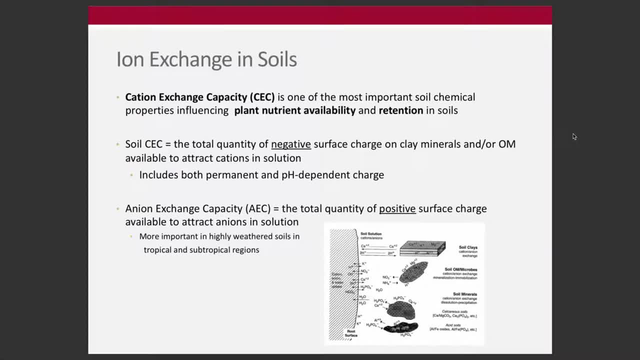 we want to keep an itemーい, a European soil running different. We want to aggre, to be on top of different can do elements in soil ninguna So country conditions can look like this. CEC or cation exchange capacity is one of the most important soil chemical properties that influence plant ingredient availability, influence plant nutrient retention. 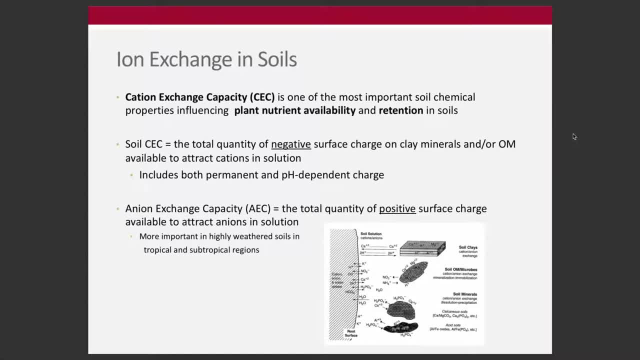 in soil. So it's often one of the- I would call it a fundamental or a foundational property of a given soil that determines or dictates what that soil is, how nutrients cycle through soil, etc. etc. Soil CEC can be directed to some soil area or waist area. or Shaq line area or continue passing through 부분이 area. This soil remained, however, inisine, зачем clamped into the soil, meaning that it liner Membery OR China bone balsam of mass and is subject to being placed into the soil. 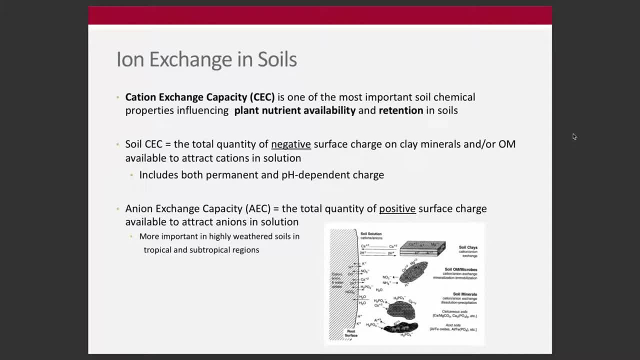 defined as the total quantity of negative surface charges on clay minerals. So the ability to attract and hold cations is really what CEC is. It's how it's defined in many ways, And so CEC includes both permanent and pH dependent charges. 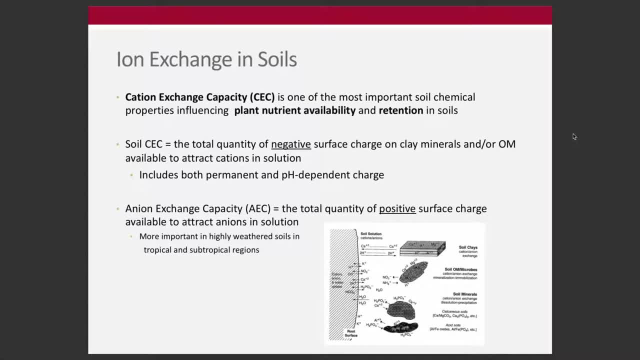 And so some of the charges that exist. what does that mean? That means that some of the charges, if we think back to intro soils, some of the charges are permanent. They're always there, regardless of pH changes, And some of the charges might flip from a plus charge. 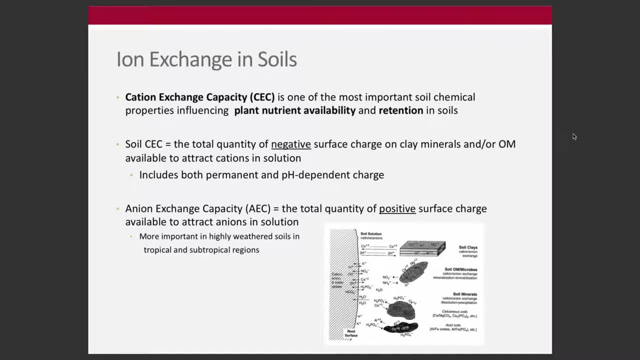 to a minus charge, depending on the pH of that soil, the pH of the solution. So we can also think about anion exchange capacity or AEC, And conversely to CEC, it's the total quantity of positive surface charges. 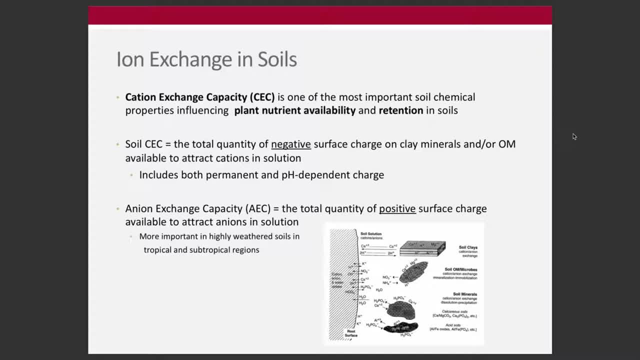 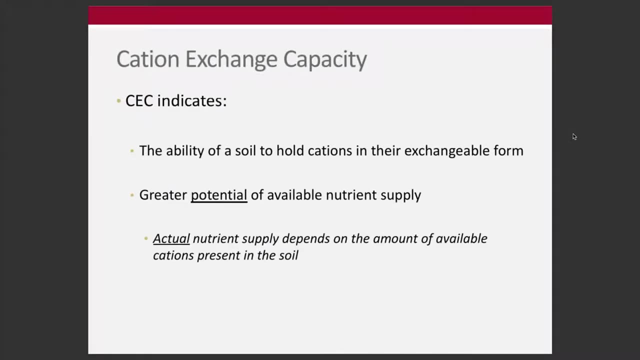 So AEC is more important in highly weathered soils and tropical or subtropical regions, But, like I said here in Ohio, CEC is by far a more important property in what we think about. So CEC or cation exchange capacity. 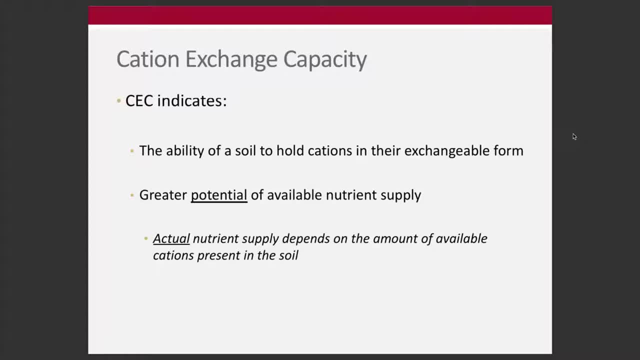 indicates the ability of a soil to hold cations in their exchangeable form. It's a measure of potential of available nutrients and nutrient supply, But it's not really a measure of the true or the actual nutrient supply. That's going to depend on what cations are there. 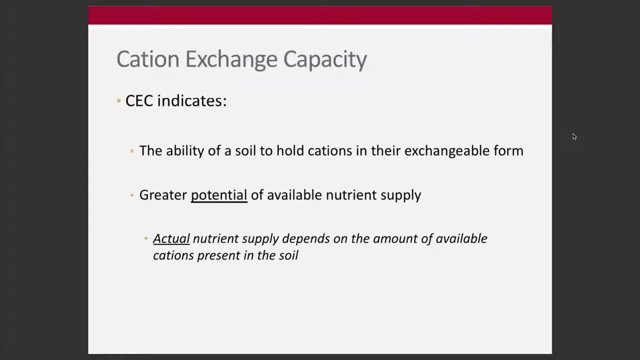 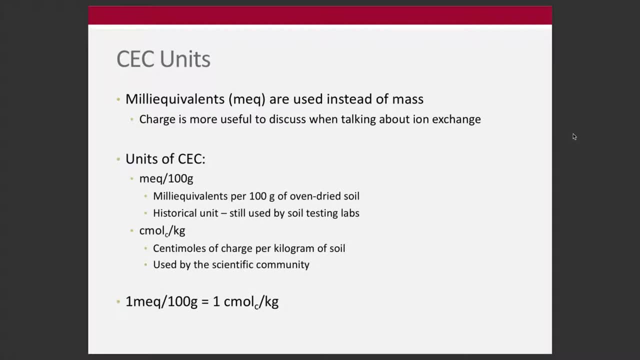 and in what proportions. That's going to depend on the actual nutrient supply, of course. OK, CEC uses a kind of a funky unit And we often mill it. It's a milliequivalent is really the standard metric. So milliequivalent per 100 grams of soil is really what's used. 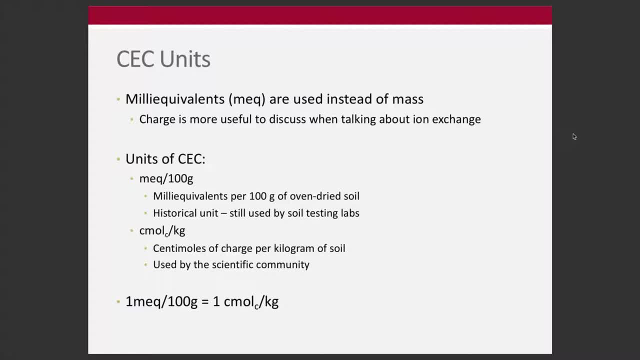 And so a milliequivalent is a measurement of charge Lots of times in soil tests and we'll get into some of this a little bit later. but when we look at a soil test it will say percent organic matter or part per million of calcium. 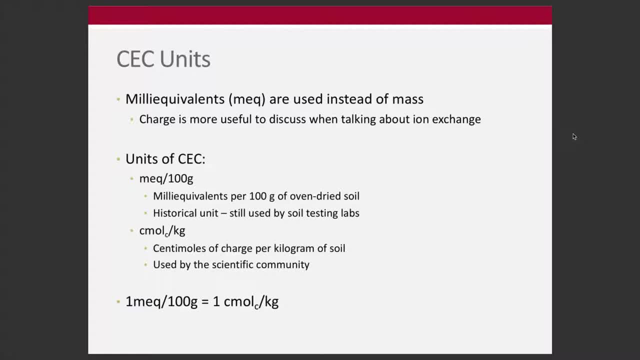 or phosphorus or potassium. Those are really mass. It's a mass of organic matter or a mass of calcium per mass of soil. So it's a measurement of concentration For CEC. we think charge is really more useful when discussing ion exchange. 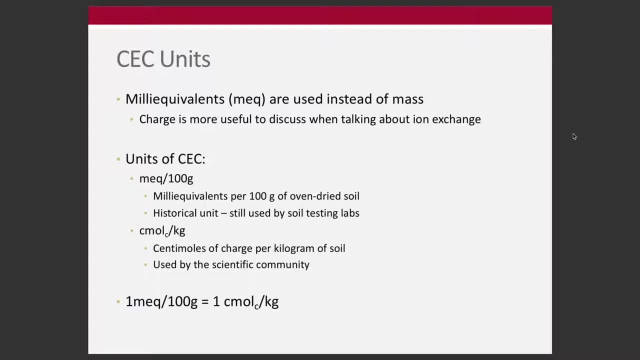 And so we use this unit accordingly. So milliequivalents per 100 grams of soil is what you'll see everywhere except in the United States, except when you're in scientific literature, And the SI unit is centimole charge per kilogram of soil. 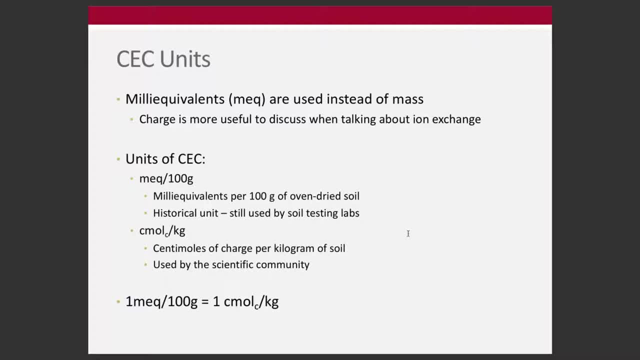 And so that's this designated here: centimole charge per kilogram. Fortunately, it's one of these rare, rare times when the kind of English or imperial unit, the one milliequivalent per 100 grams of soil, actually equals one centimole charge per kilogram. 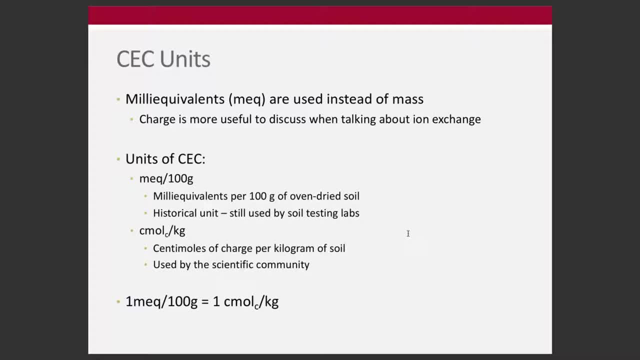 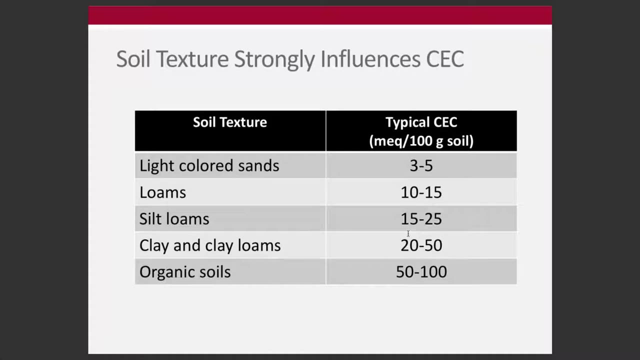 So, fortunately for us, this is one time when we can. the units might be different, but the meaning and the scale of those units are the same, So those are equivalent measurements. Mentioned that soil texture strongly influences CEC, And so this is really why CEC is an important measurement. 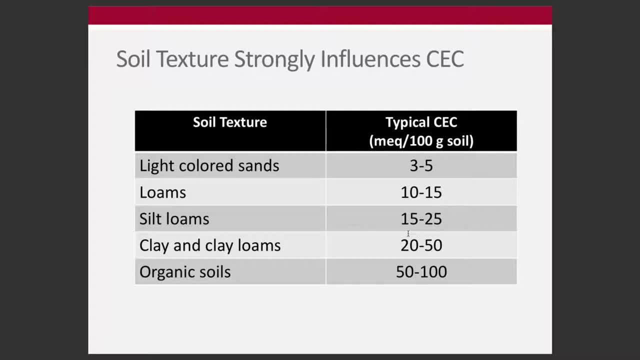 because it dictates the type or the the texture of the soil. We can see really sandy soils might have CECs of three to five milliequivalents per 100 gram, Lots of ag soils in Ohio and a lot of soils in general. 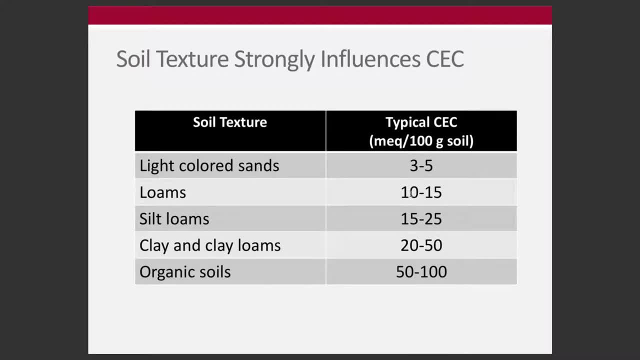 the vast majority of them will fall in somewhere between like seven or eight to 15,, up to 20.. And so those are loams and silt loams. We can have soils In Ohio that are much higher than that. So you know, CECs of 20s to 25s are not uncommon. 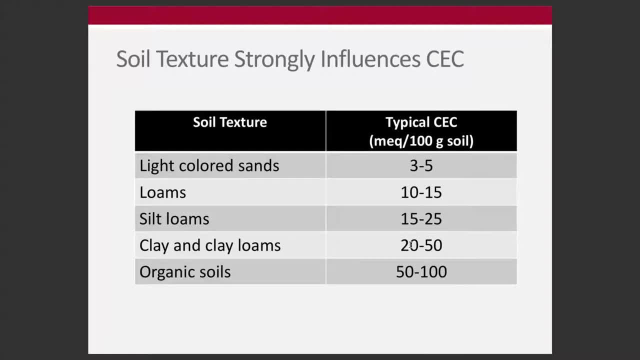 Those are getting into very clays and heavy clay soils And then soil thing CECs that are above 25, maybe into the 30s or 40s. those are really gonna be inorganic soils. Here in this table it's listed into 50 and 150 would be the. 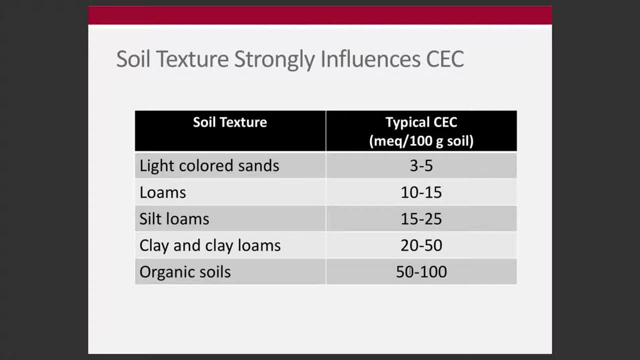 you know, if it's above 50, it's absolutely inorganic soil. but really in many cases, before much, much before we get there into the 30s or above, we're calling those organic or muck soils in general. 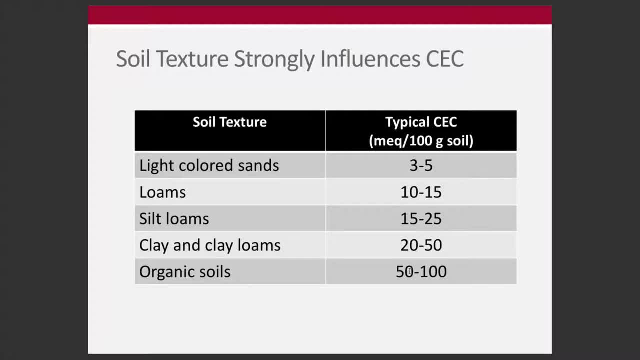 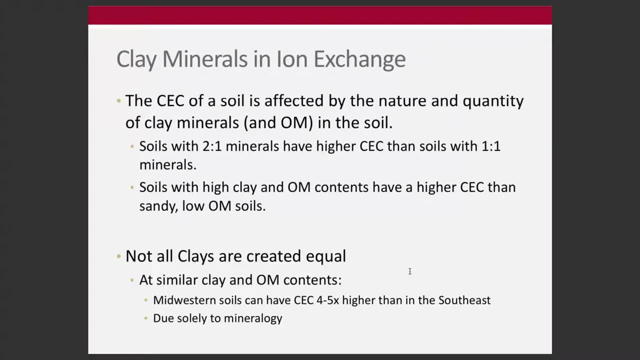 And that is because they've got so much organic matter in there that it's really driving those CECs up, okay, So CEC of a soil is affected by the nature and quantity of clay minerals- Soils with two to one minerals. 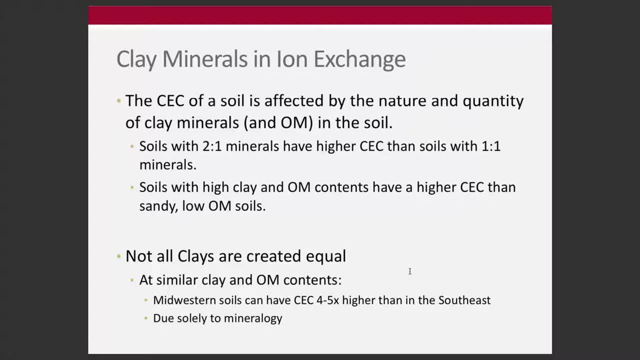 have higher CECs than soil with one to one minerals. Well, what does that mean? Well, if you think back, and maybe some people- hopefully most people in this class- have taken in intra soils, but if you haven't, it might require a little bit of legwork. 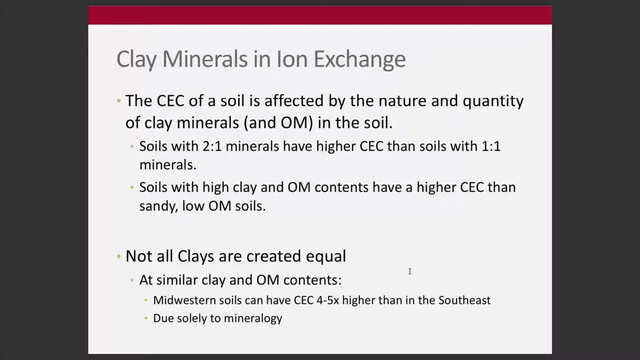 to kind of catch up to some of these concepts, And we'll talk a little bit about two to one, one to one here in a second. but soils with high clay and organic matter contents typically have higher CECs. right, We just talked about that. 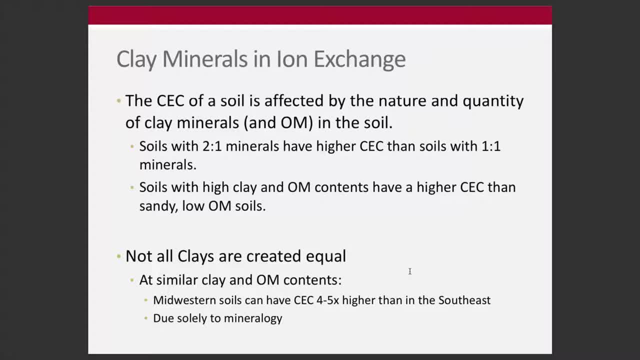 However, not all clays clays are created equal. Given similar clay contents and similar organic matter contents, soils, say, in the Midwest and in Ohio or in really most of the Corn Belt, can have much higher CECs than, say, soils with the same clay content. 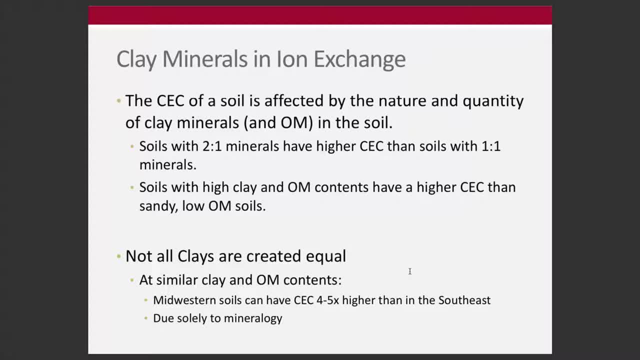 same organic matter content, say in the Southeast. What's the difference between those two soils? Well, our soils in the Midwest have been more recently glaciated and they're geologically younger soils than the soils in the Southeast. The Southeast say Georgia, Florida, Alabama. 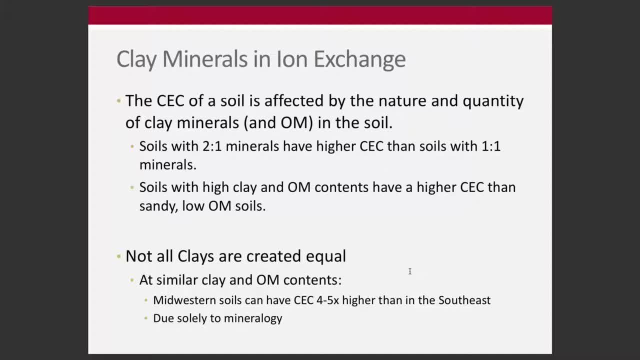 have not had recent glaciation and have had a lot of weathering. that's happened, okay, And so that weathering has influenced the type of clay, ie the mineralogy of that soil, the type of minerals in the clay and the mix of those minerals. 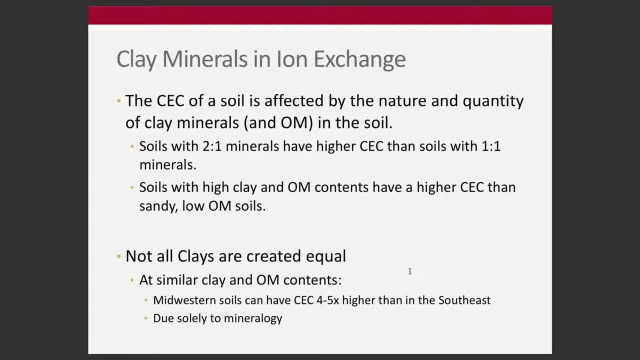 And those have different properties And typically the exchange capacity of those clays- those older weathered soils- is lower. So when we say two to one clays, those are what I'm referring to as more commonly, more recently glaciated, more fertile soils. 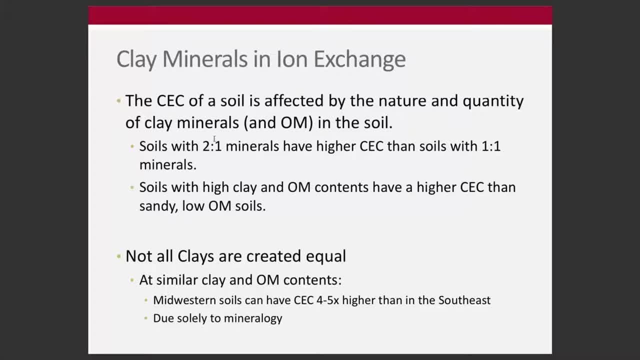 and one to one clays. So these would be things like alphasols and molasols and septasols that we would find in Ohio, in the Midwest, And these one to one clays are more oxasols and altasols. 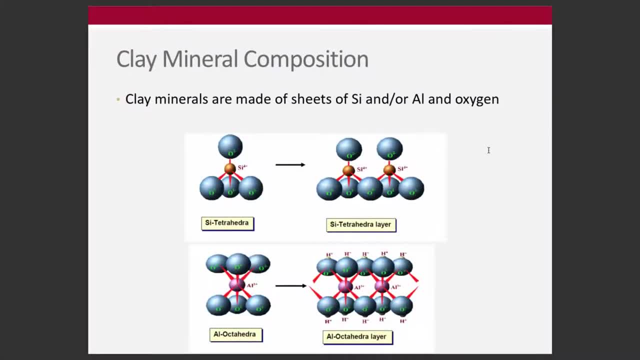 that we would find in the Southeast, okay, So we're gonna pick this apart and you're just gonna have to bear with me for just a few minutes while I get into some of the nitty gritty. And I think this is you know. 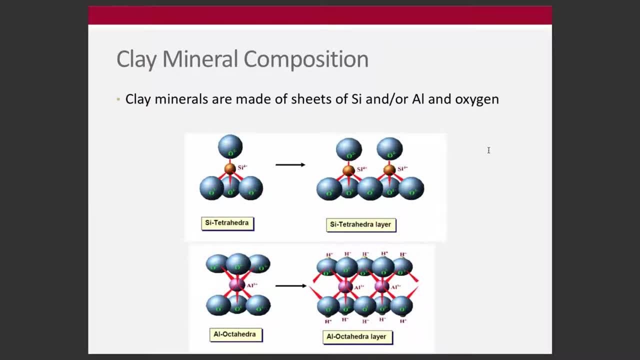 it's important really to kind of understand some of these concepts. when we're talking about two to one and one to one, what are we talking about? Okay, so clay structure, clay mineral. this is greatly simplified. You know, mother nature is a complex beast. 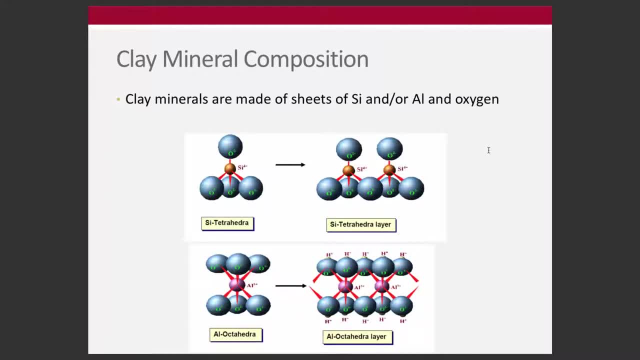 but let's just talk about it. from this We forgot either clay is really made up of- and this is you know from Soil Science 101.. You know, pull your Brain Wild book and you'll find this, but they're made up of oxygen and silicon. 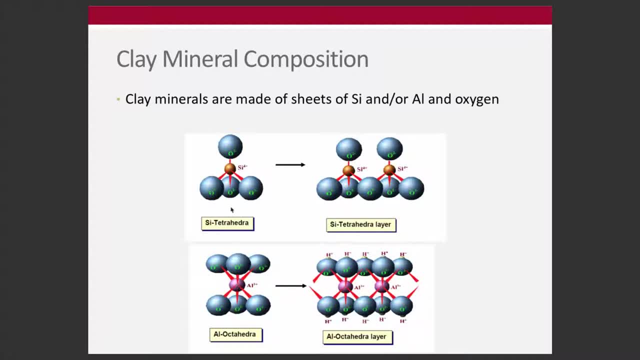 or they're made up of oxygen and aluminum, right? So these sheets of silicon tetrahedral sheets are aluminum octahedral sheets. okay, So there's here. there's a silicon with one, two, three, four oxygen, And here there's aluminum with either six or eight. 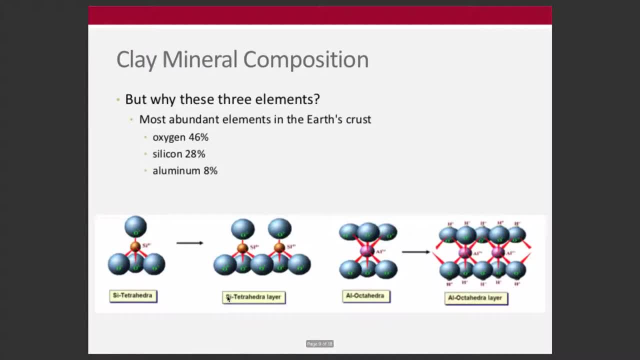 making this octahedral sheet okay. And so why these three elements? Well, not surprisingly, if you look at kind of the entire composition of the Earth's crust: oxygen, aluminum and silicon make up a large percentage of the total amount of you know of Earth, right? 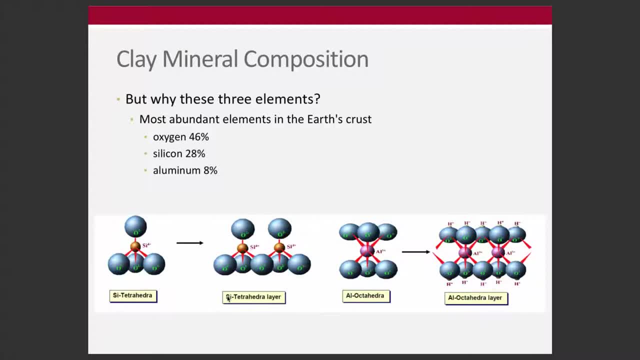 That's well, in the crust of Earth at least, And so there's a large percentage of these three things and that's, you know, that's the stuff dirt is made of, soil is made of, right, So, but getting back to this idea of one-to-one clays, 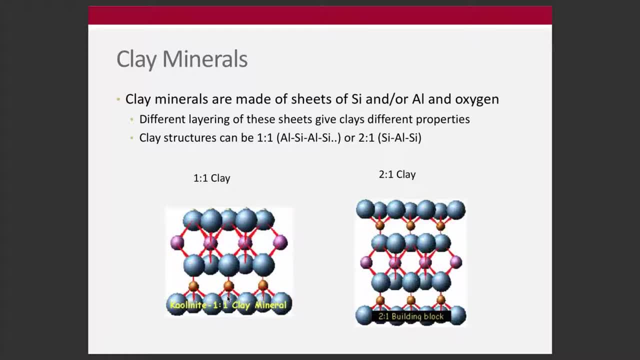 versus two-to-one clays. that designation is a generalization for clay and it depends on if it's one-to-one of these octahedral and tetrahedral, these aluminum and silicon sheets, or if it's a silicon- aluminum- silicon sheet. okay, 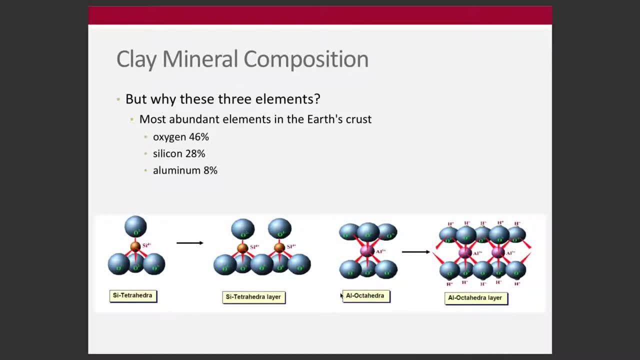 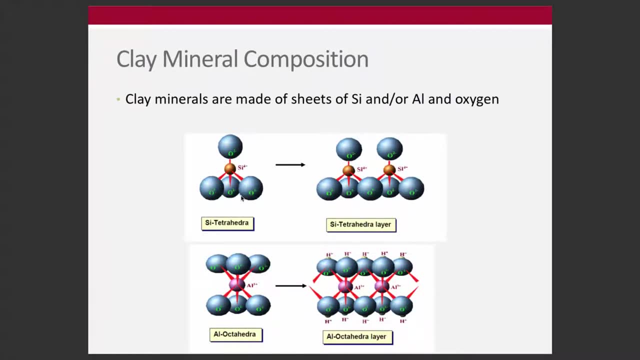 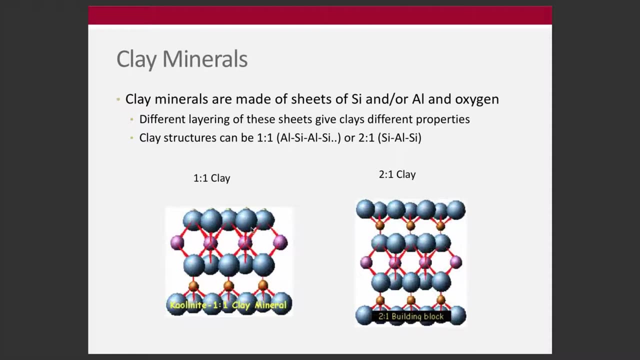 So again going back- and I realize this isn't the greatest pictures of all time here, but we've got these silicon tetrahedral and these aluminum octahedral, and that really determines the alignment and arrangement of these sheets, if it's one octahedral to one tetrahedral. 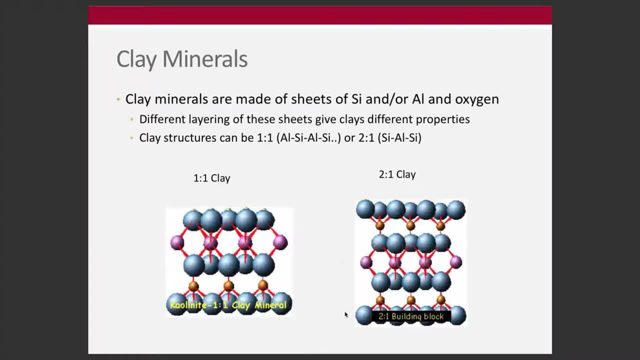 or if it's one tetrahedral to one octahedral to one tetrahedral. So one-to-one, these two different types, or one-to-two-to-one, or sorry, these two-to-one. so there's for every one octahedral. 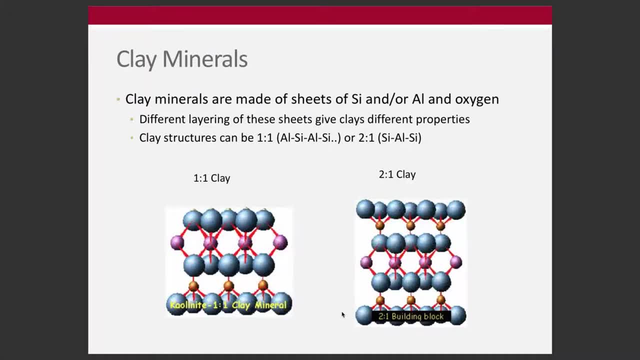 there's two tetrahedrals, okay. So, anyways, that is really kind of what we're talking about and thinking about. You'll hear, you know, kind of in the soil, science literature or even in practitioners talking about- oh, those are mostly one-to-one clays. 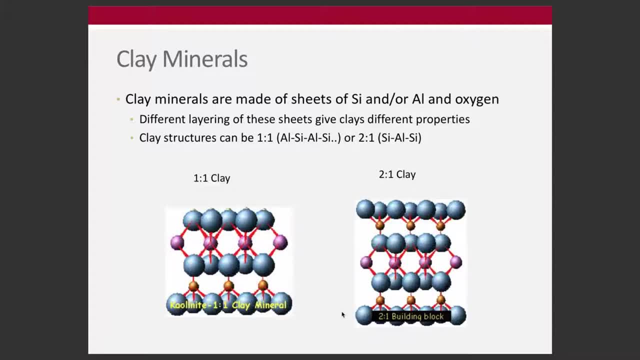 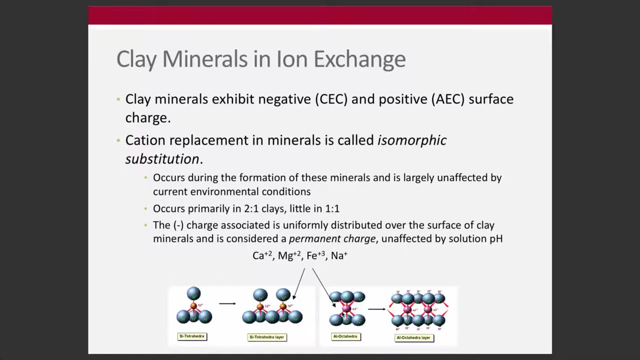 or these are two-to-one clays and this is really what they're talking about, And a lot of this is dictated by the type of mineral and the weathering of that mineral in the formation of that soil. okay, So if we think about this- I told you before- 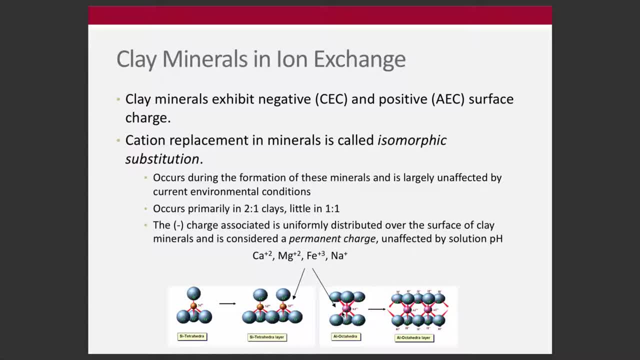 that one-to-one clays can have a lot lower exchange capacity than these two-to-one clays. okay, And so why might that be? Well, it's primarily because of a process called isomorphic substitution. Again another soil science 101 term. 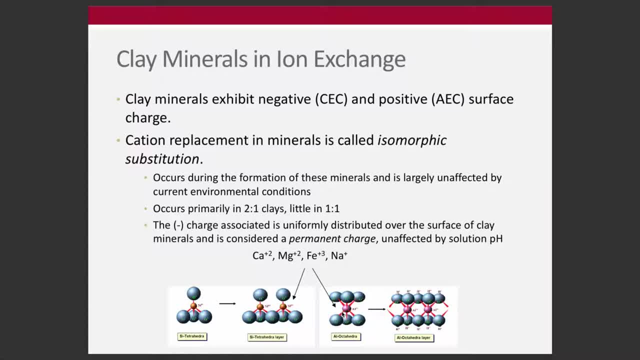 And all that means is, over the course of millennia, right weathering of these soils. you know, on the orders of thousands of years, tens of thousands of years and maybe even longer, hundreds of thousands of years, we have a lot of water moving through the profile. 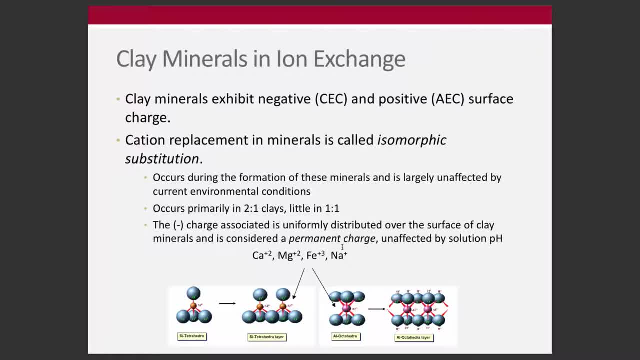 a lot of interactions, of the ions that are in soil, And sometimes this silicon, this plus-four silicon or plus-three aluminum, gets substituted out with other cations, right, And so if one of these cations a plus-two, plus-two, 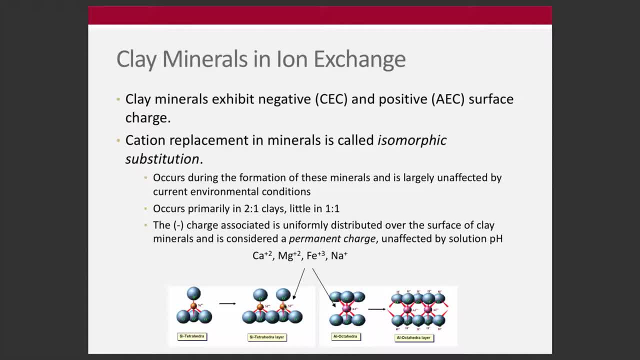 plus-three or a plus-one exchange for this plus-four silicon or this plus-three aluminum. at best we're substituting the plus-three iron, but at worst we're losing actual plus charges. okay, And so the longer, the older a soil is. 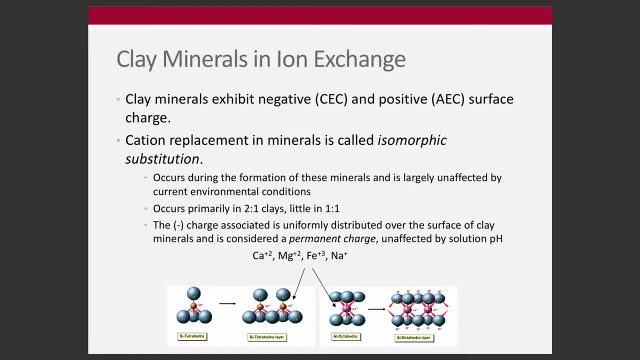 typically the more of this isomorphic substitution. that is a one-to-one substitution but it's got actually a lesser charge And that results in actually a net reduction of permanent charge in the soil. okay, So that's really kind of what we're talking about. 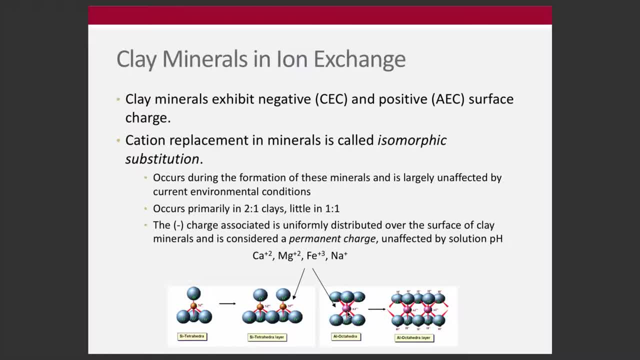 And this is just. like you know, this isn't information that you're going to use every day, but it's just a good foundation to kind of understand what people are talking about with CEC. two-to-one clays. one-to-one clays. 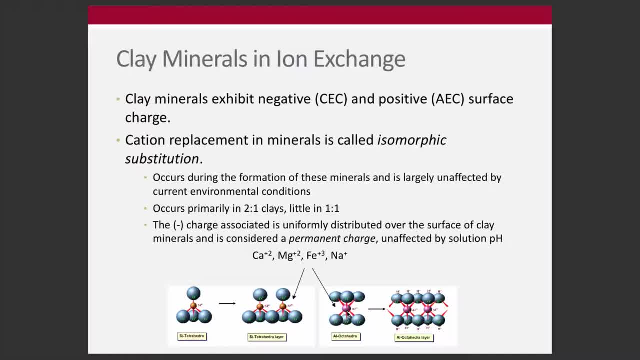 There's a process And a lot of this is determined not by our management and what we do, but it's determined by how young those soils are, how recently glaciated, how you know. it all goes into kind of all the soils in the Midwest. 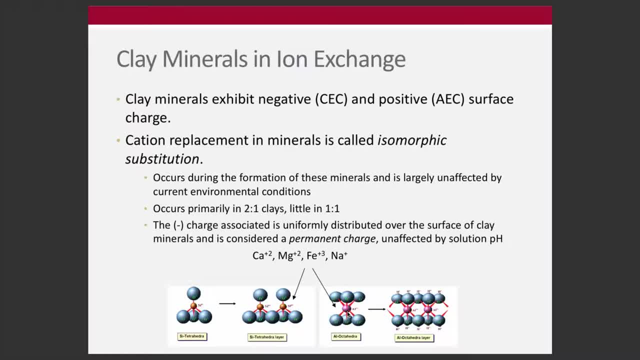 the Corn Belt are really fertile soils. You get down to Alabama, Mississippi, Georgia, and those soils aren't nearly as fertile. Well, why is that? What does that mean? Well, part of that is because of these mechanisms right here. 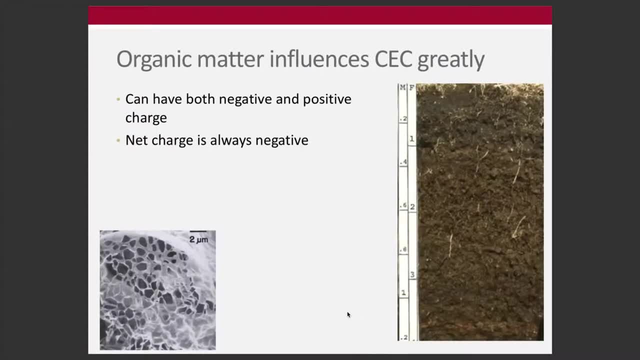 okay, All right. So let's kind of come back to the surface here. Think about organic matter. I mentioned that organic matter greatly influences. We already talked about. we'll talk a lot more about this as the course progresses. Organic matter represents a small fraction. 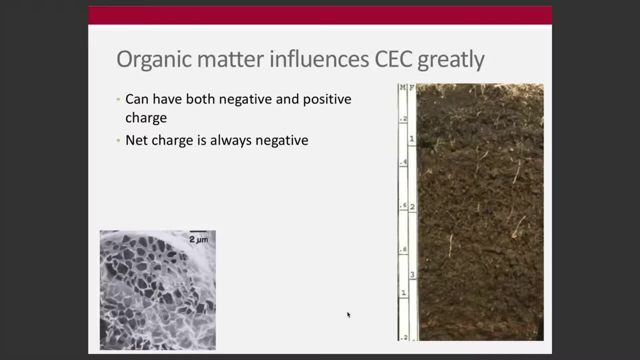 of the total soil but again plays a very disproportionate role, And it's certainly true with ion exchange and CEC. So a small amount of organic matter. you know, if you go from two to 4% organic matter in a soil, or from four to six or something. 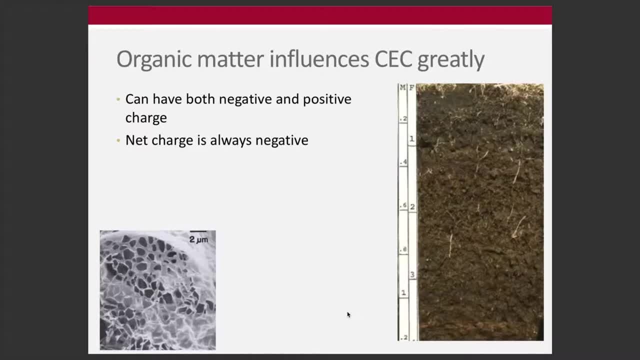 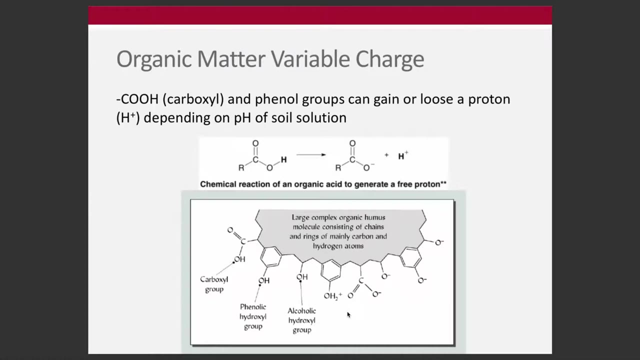 you can increase your CEC greatly because of that. So it really increases the amount of exchange sites, the ability of that soil to hold nutrients, And that's why building organic matter is such a key piece of building a soil's fertility. And so there's these carboxyl and phenol groups. 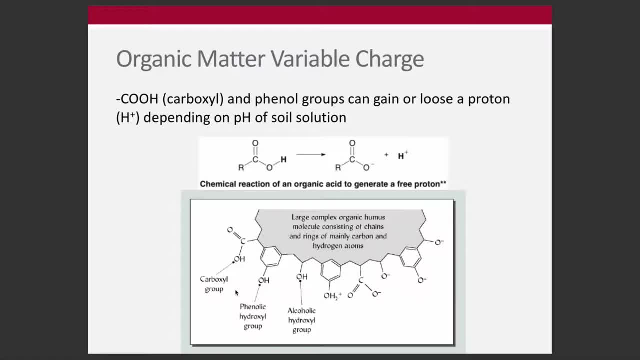 all kinds of stuff. you know These are the common ones- carboxyl groups and phenolic groups that are able to. you know they disassociate with hydrogen and then it leaves this negative charge. So then, say, calcium or potassium magnesium. 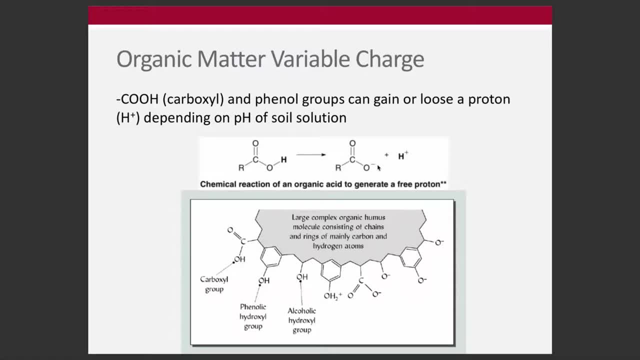 something comes and attaches here And then that is essentially an ion, a nutrient that is able to be plant available. okay, So this is again a couple of the mechanisms with organic matter. We, anytime we talk about organic matter, we need to realize it's incredibly chemically. 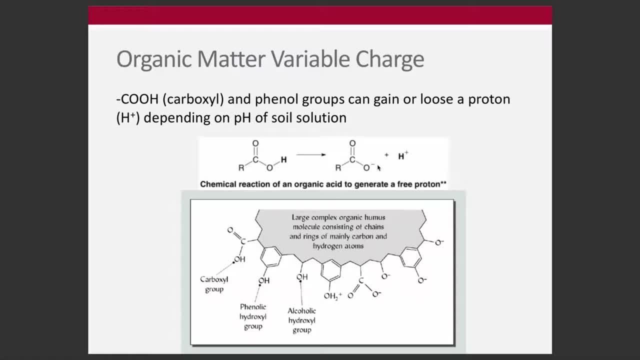 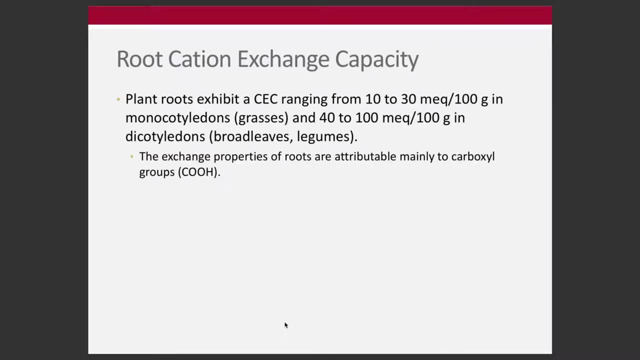 complex and it's very difficult to kind of generalize across this, But here are two commonly occurring organic compounds, organic groups- this carboxyl group and this phenolic group- that exist. okay, Roots are made up of organic matter and, as such, 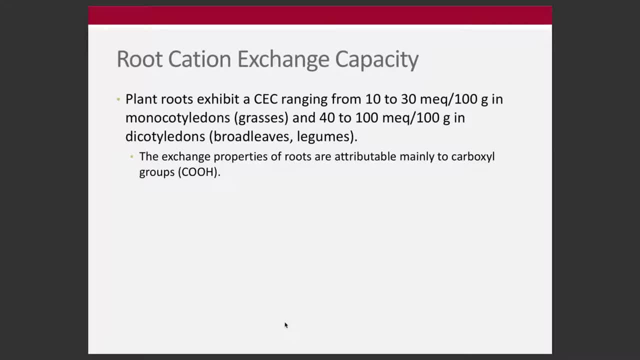 they play again a disproportionate role in ion exchange and CEC. And so you know these. you know monocotyledons, like grasses, are typically a little. you know grasses often have much more root mass, a lot of fibrous kind of roots. 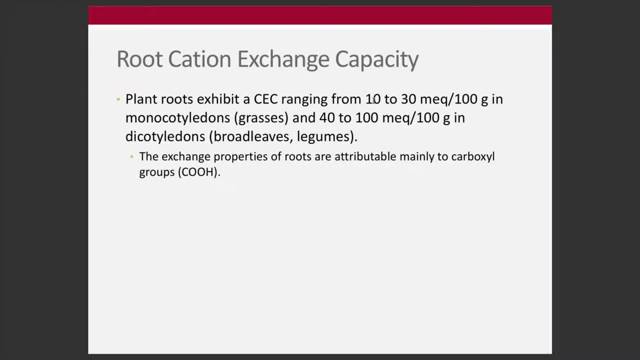 But because of that, or partially because of that, they contribute maybe a little bit less to the CEC than things like dicots, like broadleaves legumes et cetera. So you can see the magnitude of CEC contribution. 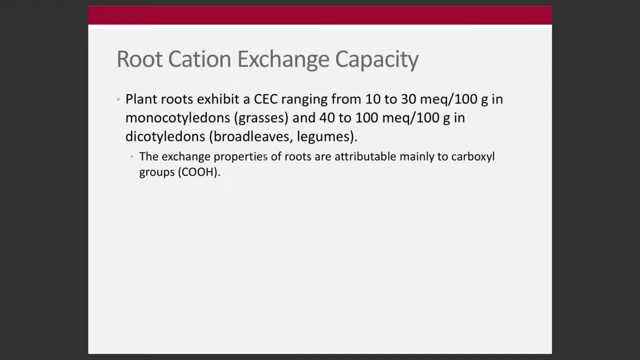 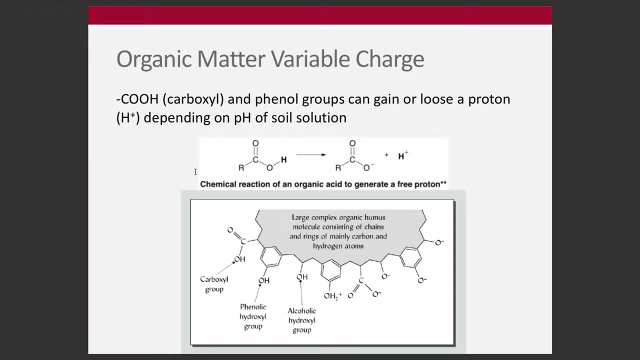 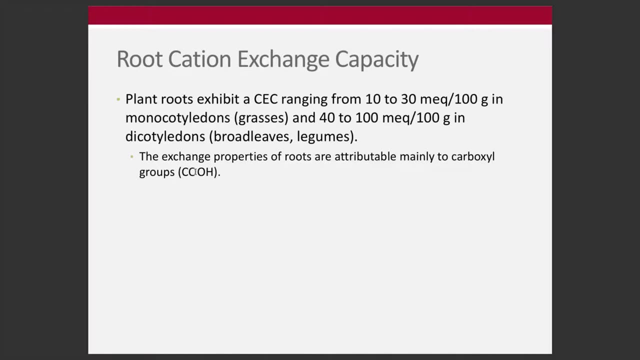 10 to 30 versus 40 to 100.. Okay, And again, you know, not surprisingly, organic matter is primarily derived from root sources, from plant material, And so these are the same kind of exchange properties, the same types of organic compounds. 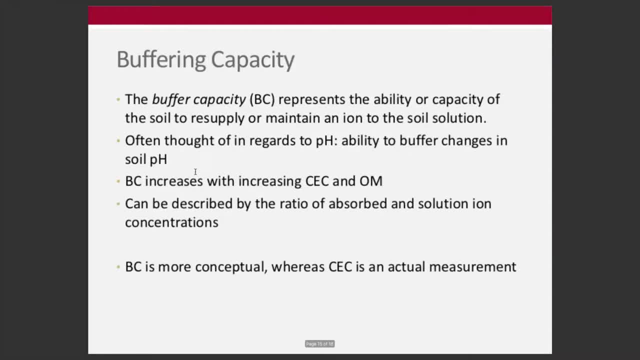 that are contributing in organic matter, as in live roots. okay, Buffering capacity is another concept. We don't really measure this, like in a soil test, for example. there's ways to do that, But it's not commonly done. But it's more as a concept that represents the ability. 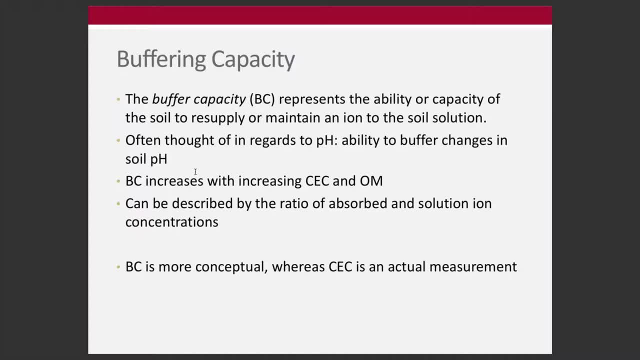 or capacity of a soil to resupply an ion. So in the last lecture we talked about plucking, plucking nutrients out of that soil solution. Buffering capacity is a concept that describes the ability of that soil to resupply that soil solution with the ion. 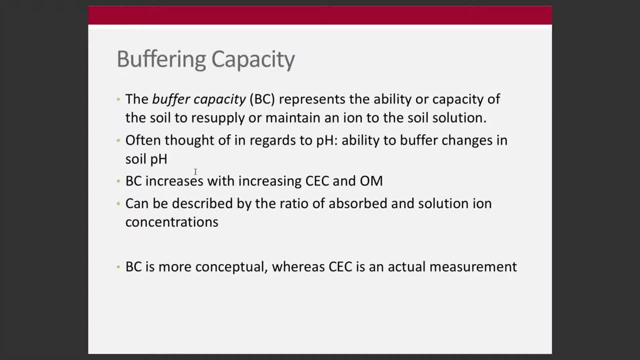 that was taken up by the crop or lost via leaching, or lost via, you know, atmospheric losses or what have you? okay, So it's often thought of in regards to pH, So how you know, when we talk about buffering. 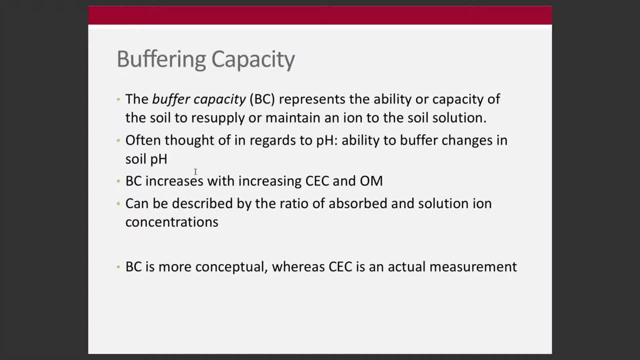 it's the ability to resist changes, And pH is an important piece of this. But we can think of buffering capacity in the context of pH and acidity. We can think of it in the context of nutrient supply. But both times, in both scenarios, buffering capacity of a soil will increase. 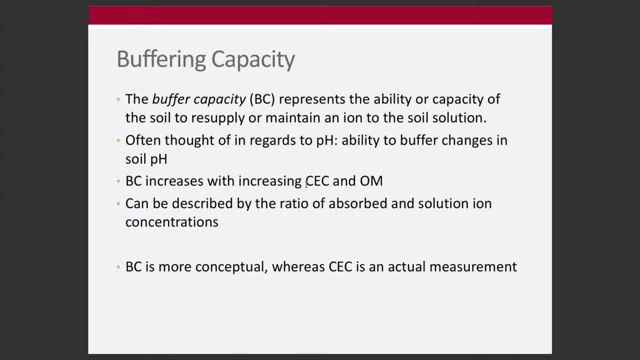 as CEC and organic matter increase. okay. So at this point you get asked the question: well, the more CEC I have, the more organic matter I have, it must mean it's a better soil, right, Like? and typically the answer to that question is a little bit. 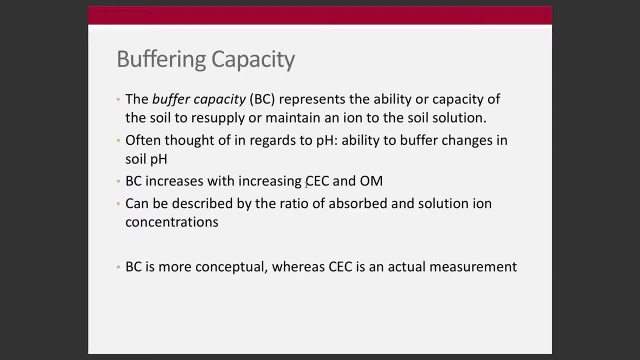 tricky. you know it depends a bit. But as your CEC increases, your clay content will often increase And you can get into really heavy clays that wouldn't be considered the most fertile soil of all time. So there's caveats, you know, with this. 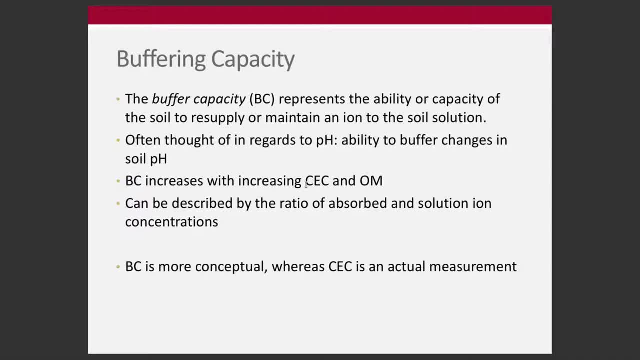 But anyways, buffering capacity again is an important concept to think about. When we do something to a soil, we you know if we're influencing the pH or influencing nutrient availability, how, what is the ability of that soil to resist? 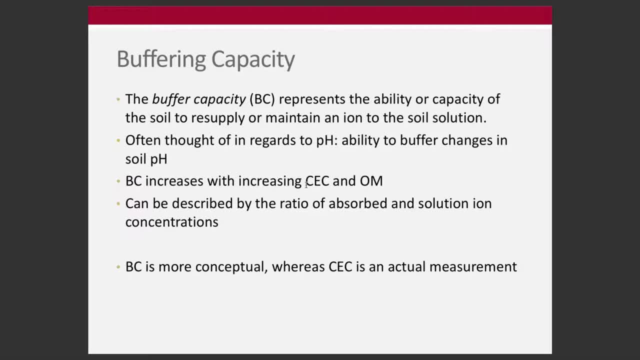 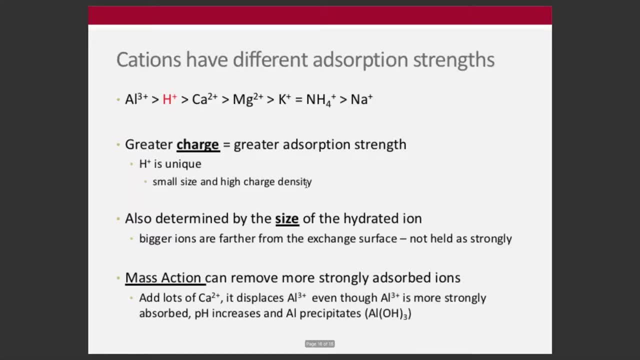 to that change. Okay, so in some ways we can think about soil resiliency and buffering capacity in kind of a similar way, although those two things are certainly not the same. Okay, cations have different adsorption strengths, And what does that mean? 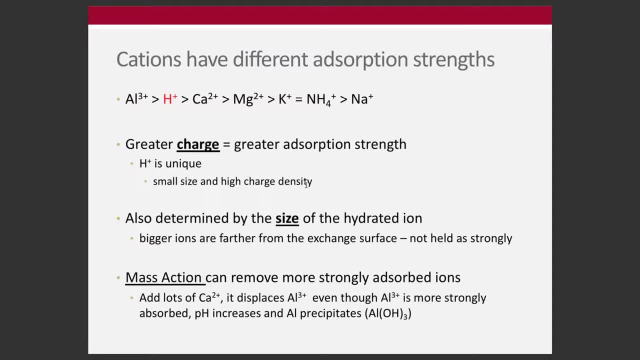 So the ability of an ion to essentially stick to the soil. it's how you can think about it. We've got a negative site on a clay surface. How does that clay prioritize? Who's on it, Who's on the VIP list or who's not? 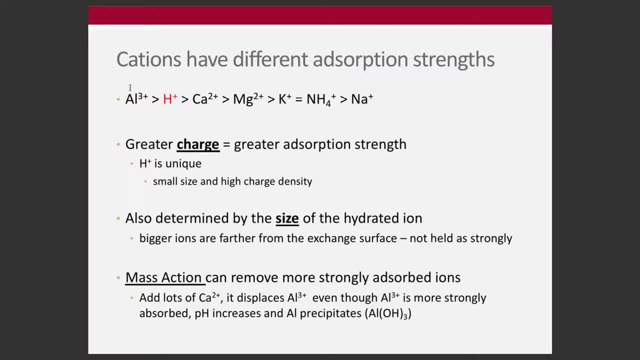 Of course, it's not really prioritizing per se, but it has to do with the chemical properties and the adsorption strength. So aluminum has a very strong adsorption strength, followed by hydrogen, by calcium, magnesium, potassium, and which is similar to ammonium. 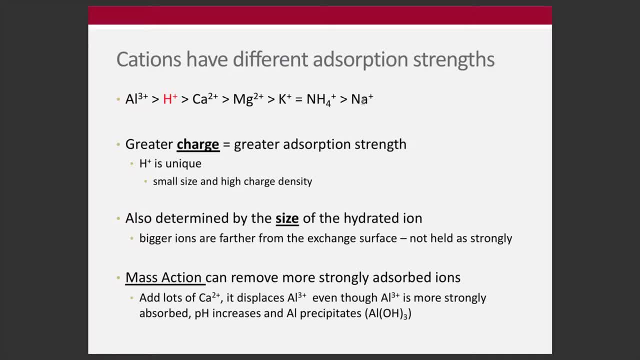 And then sodium is the least along the line And you can see, As a general rule, as we go down this gradient of strongest adsorption strengths to the least strong, our valence or our number of charges essentially changes from plus 3 to plus 2 to plus 1.. 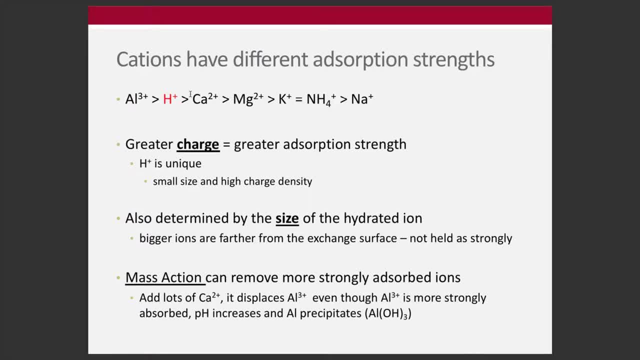 The difference, however, is the outlier. here is this highlighted in red: this hydrogen. And hydrogen is different because it's got a very small hydrated radius And so the size of that hydration radius, ie the size, the physical space that that ion occupies- 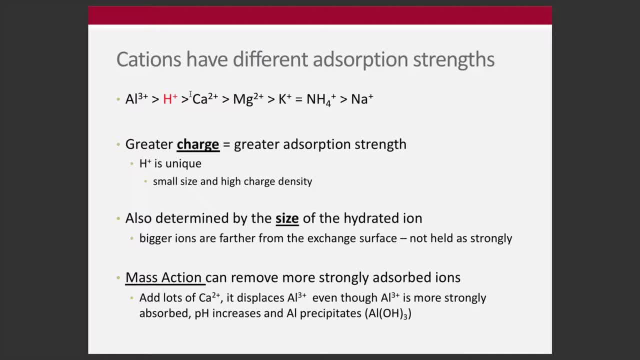 when it's in water, depends on the atomic properties of each one of these ions, And so for hydrogen it's very small, And so because of that, it's held very tightly, And so something like sodium. Sodium has a very, very large hydration radius. 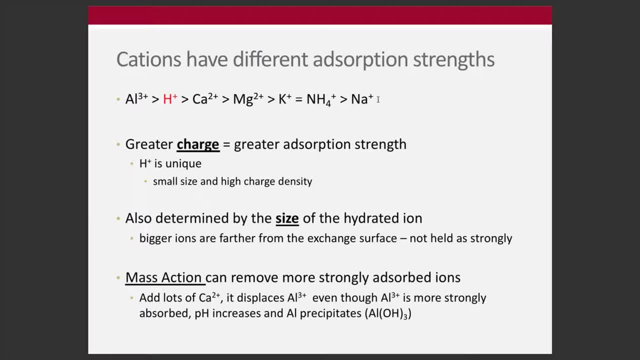 And so that's why sodium is held so weakly to the exchange site. So this slide is really just to kind of show that ions- or at least to relay that ions- aren't held in the same regard or they don't all stick to the soil at the exact same strength. 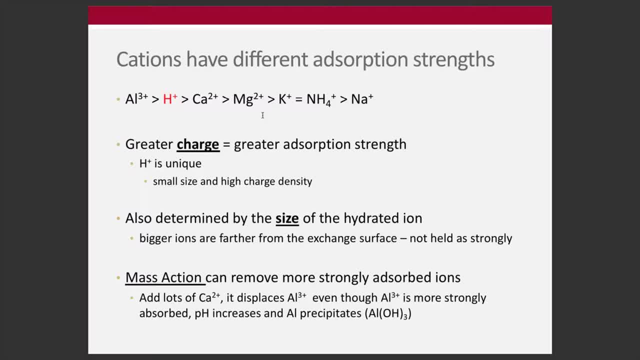 The stickiness. you can think about it like a magnet. the strength of the magnet is not. you know, some magnets are weak, some are strong. Well, here are the strong magnets and here are the weak magnets down here. okay. 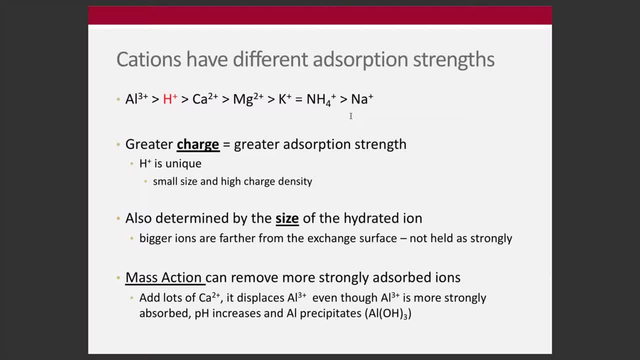 So in some ways that helps determine how much of the ion is on an exchange site at any given time. However, it's more complicated than that. not surprisingly, We talk about this concept of mass action can remove more strongly adsorbed ions. 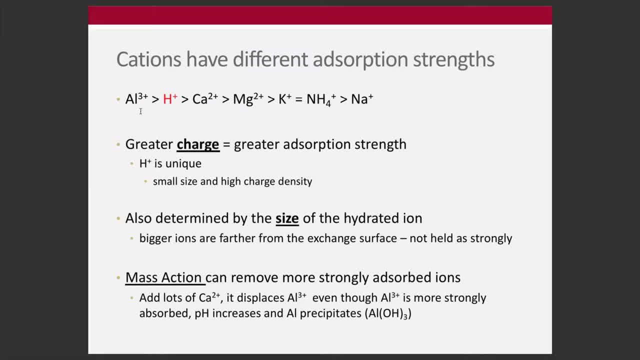 And so In the context, you know, we look at this and we say, oh well, aluminum and hydrogen, these are both acidic cations And so that's bad because that's going to drive our pH of our soil down tremendously. 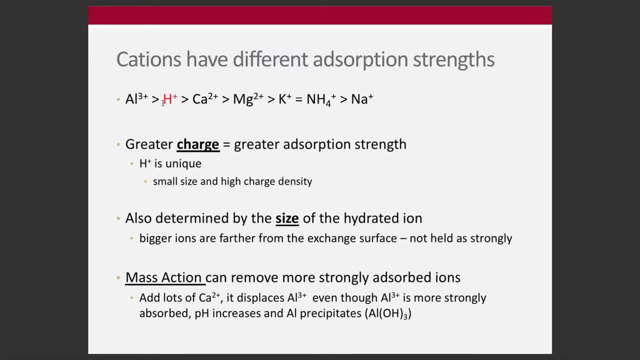 Well, the good news is that if we lime a soil, if we add a bunch of calcium on it, we can, by kind of the sheer numbers, flow off or remove, exchange calcium for aluminum and calcium for hydrogen. Because of this idea, of this mass action, you know. 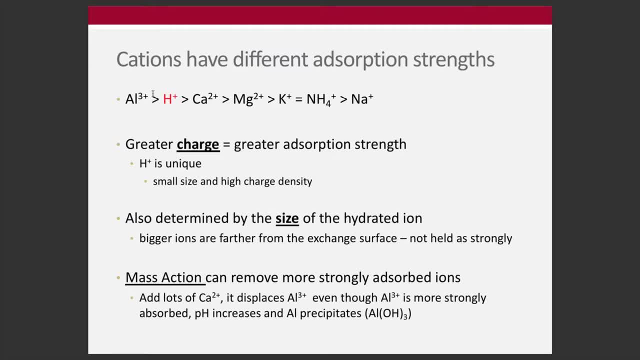 it's flowing these cations off the exchange site. So if we lime, we're adding a lot of calcium and that helps alleviate. it raises the pH, helps alleviate some of the drop in pH from these acidic cations. okay, So there's a number of pieces that are going into. 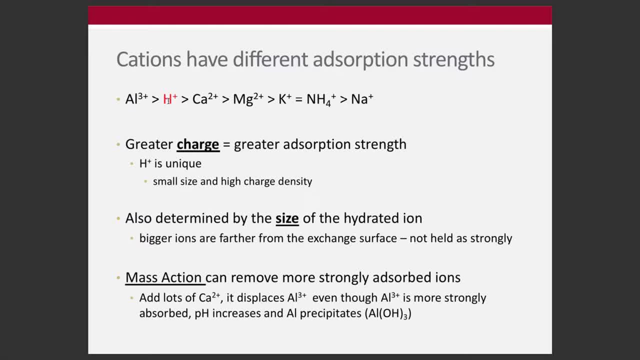 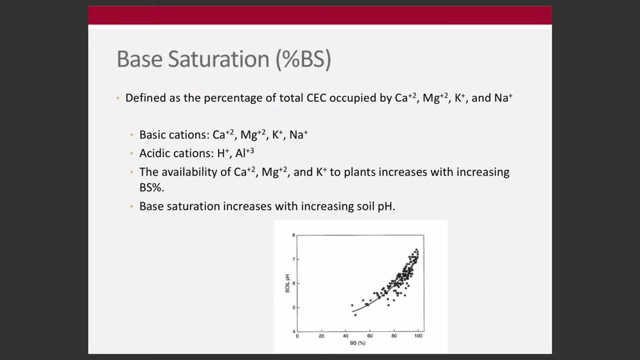 what cations actually physically exist on those exchange sites and what determines if they stick around or if they're actually leached out or moved off or, you know, immobilized or like moved into the soil solution, for example, Okay, base saturation is defined as the percentage. 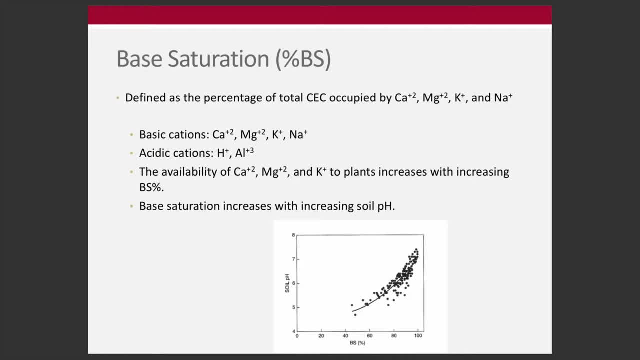 of total CEC occupied by calcium, magnesium, potassium and sodium. What's special about these four cations? Well, these are called base cations or basic cations, because they drive the pH of soil uh up. We have acidic cations, things like hydrogen and aluminum. 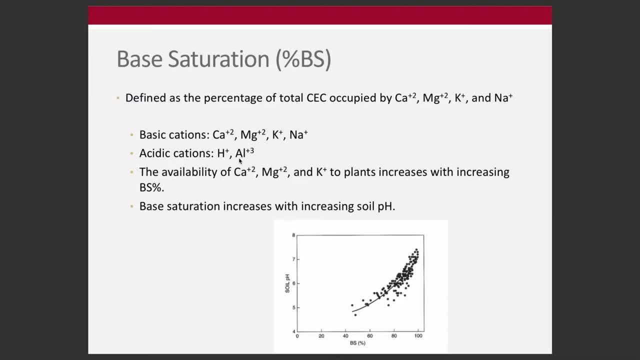 things like um iron, for example, manganese, that drive the pH of that soil um down, So it's they make it essentially more acidic. So base saturation is highly related to the pH of the soil As our base cation increase in the soil. 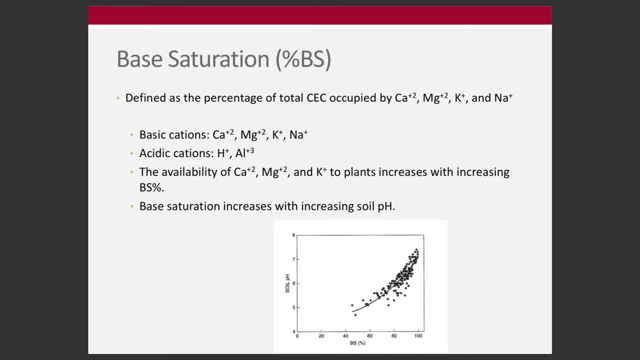 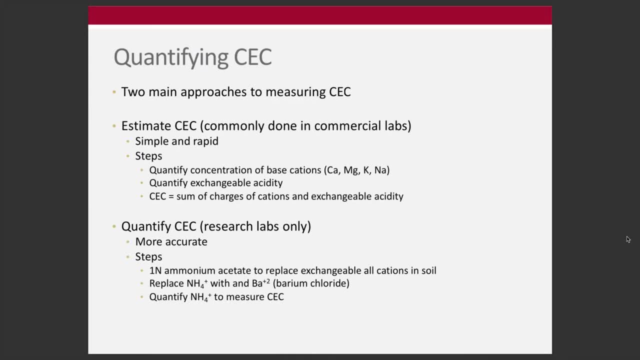 our soil pH by default increases. That's just, uh, shown here, Okay, Um, and talking about how do we actually measure or quantify CEC? well, there's two different ways. uh, that it's done. two main approaches. 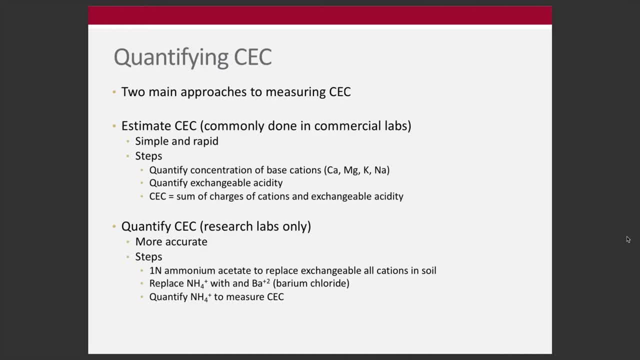 Okay, so the most common way is to really estimate it. It's a simple and rapid technique And it's really, uh, summation of the cations. So it's, you're actually adding up the cations And I'm going to post another video. 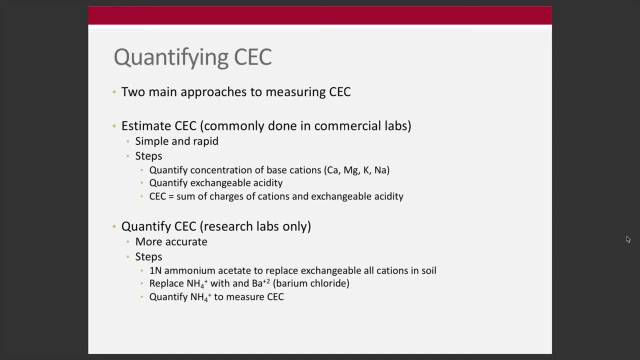 that's kind of going to dive a little bit deeper into that. And then there's a second way. that is not done very often, at least in the commercial setting. It's really done in soil research labs or whatever, But it's. it is far more accurate. 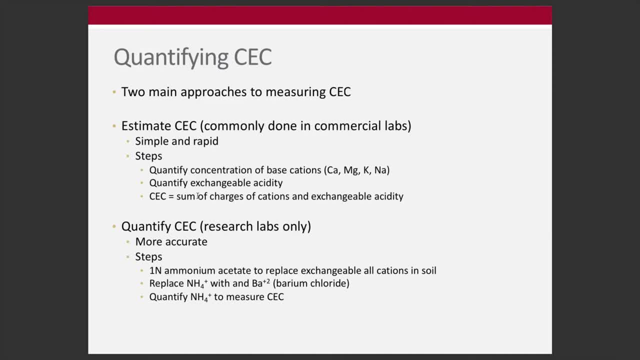 And sometimes not all the time, but sometimes this kind of this estimating CEC by summing cations, uh will fall apart depending on the soil or depending on the, the pH or the situation, But the really the, the, the kind of 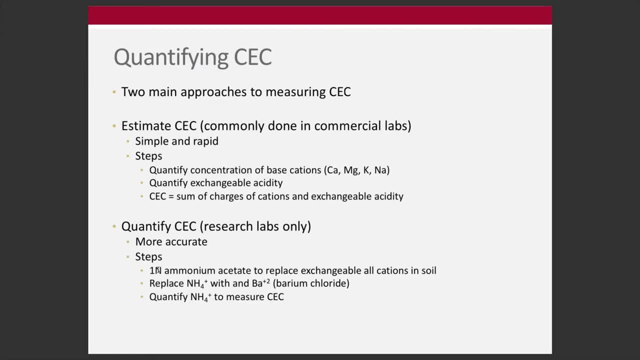 the gold standard way to quantify CEC. is this? this um done in a commercial lab where we're taking ammonium acetate and we we flood the soil with ammonium It. it it displaces all the cations. 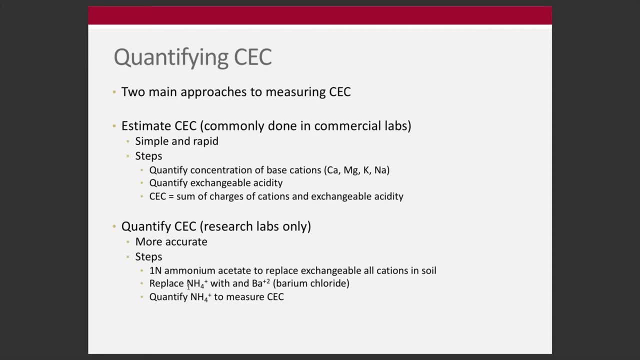 And then, uh, we take in a second step: we flood the soil with this barium chloride and it displaces all the ammonium, And then we quantify the ammonium. So it's basically like, uh, physically, um, removing, you know. 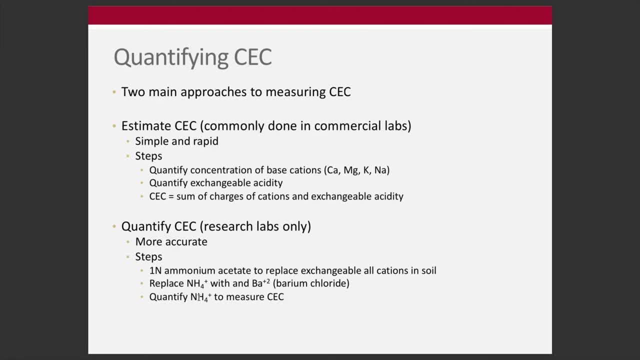 all the cations except for ammonium, And then we're quantifying ammonium. So this is anyways. uh, there's a little bit more about this in soils, textbooks or you can. you know references online, But this is not a test. that's done that commonly. 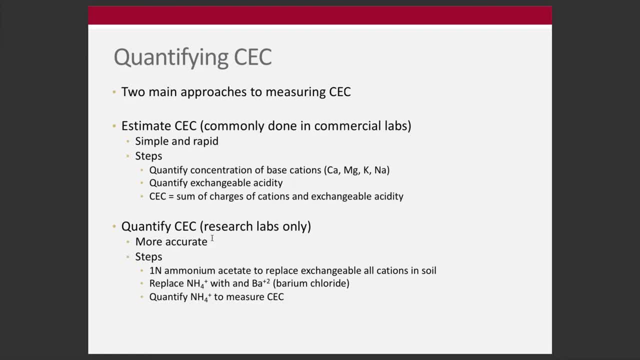 except for maybe in a soil characterization lab. This uh sum of cations is is much more common. So again, we'll we'll wrap up here and then we'll I'll post another video going a little bit deeper into that.